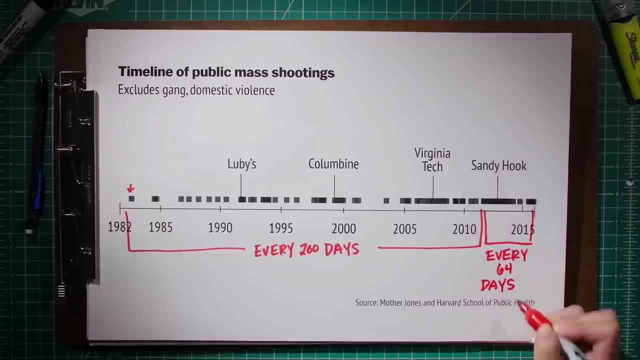 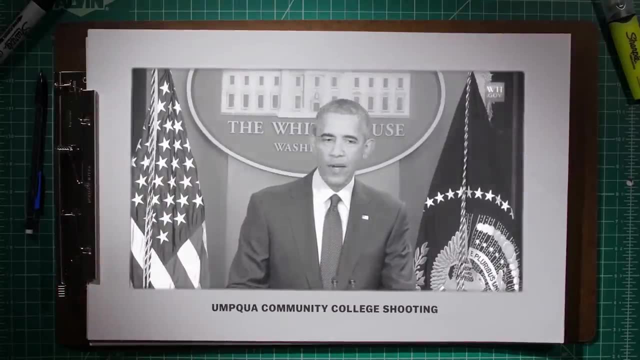 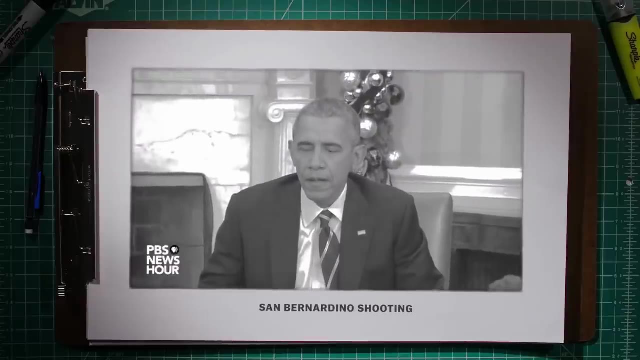 I hope and pray that I don't have to come out again during my tenure as president to offer my condolences to families in these circumstances. That was October 1st 2015.. And just about two months later, Yesterday, a tragedy occurred in San Francisco. 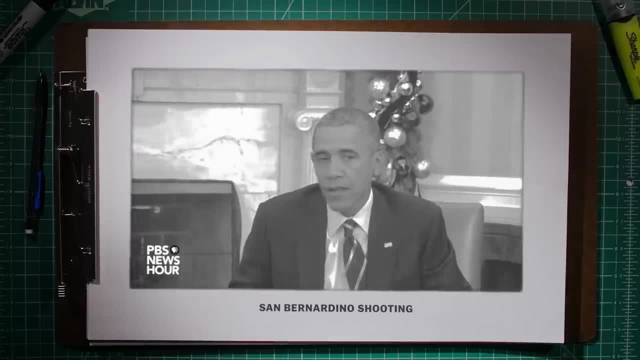 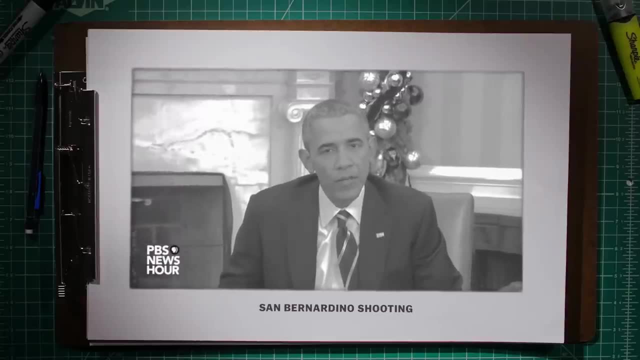 We learned. our first order of business is to send our thoughts and prayers to the families of those who've been killed. Public mass shootings get all the attention because they're often so indiscriminate, But the truth is mass shootings are unlike most gun deaths in America. 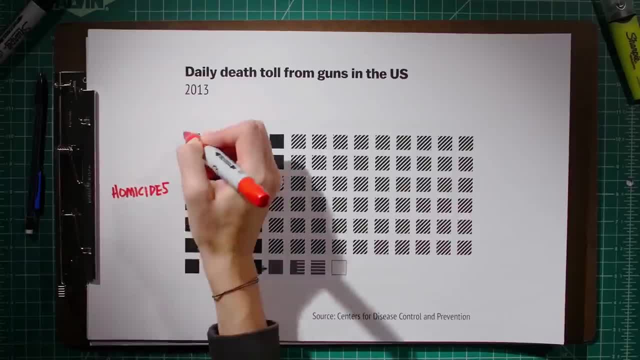 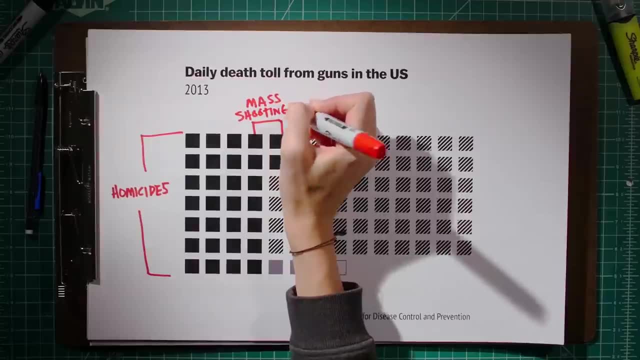 Here's how it breaks down. According to the most recent data, 92 people are killed with guns every day on average. About 30 of those are homicides, of which maybe one and a half at most can be considered part of mass shootings. 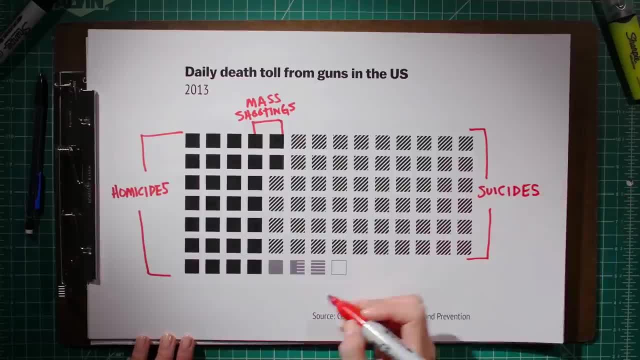 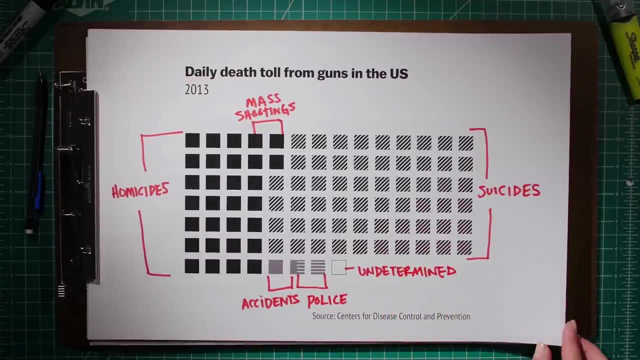 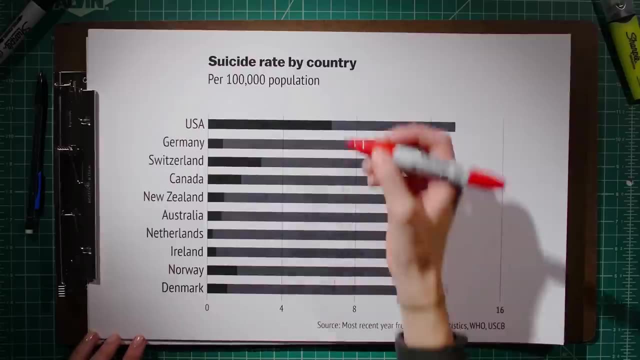 Of those killed, 58 people a day are suicides. The rest are accidental shootings, police actions and undetermined incidents. Those suicides- they show up in international comparisons too. These are the 10 countries ranked highest on human development by the UN. 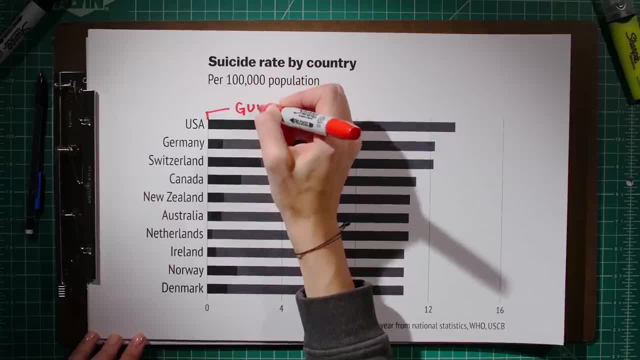 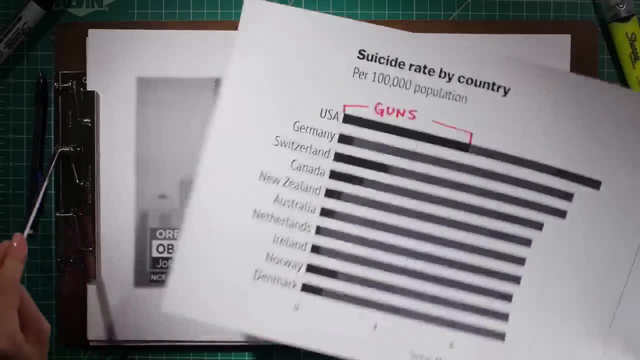 The US has the highest suicide rate among them, And this darker bar shows how many of those are. with guns, Some people think suicide isn't really relevant to the gun issue. I think that some type of gun control regulations that are being talked about are going to stop somebody from committing suicide. 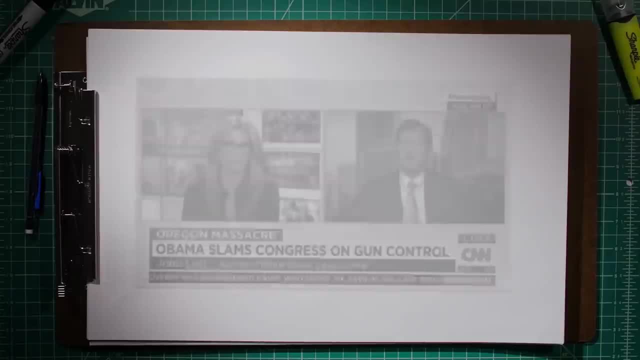 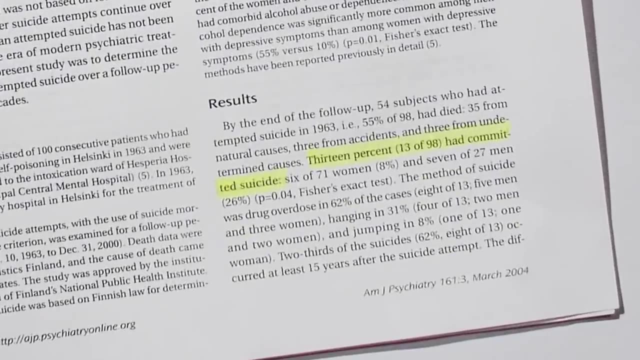 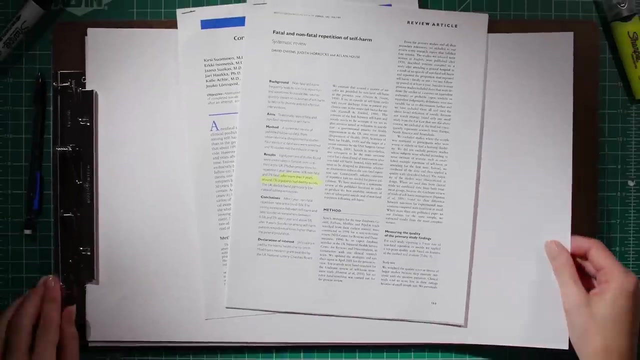 when there's so many other ways for people to commit suicide. But the methods that people use are important, because suicide attempts often stem from temporary crises. The vast majority of people who survive suicide attempts don't end up dying from suicide, But guns make it nearly impossible to get that second chance. 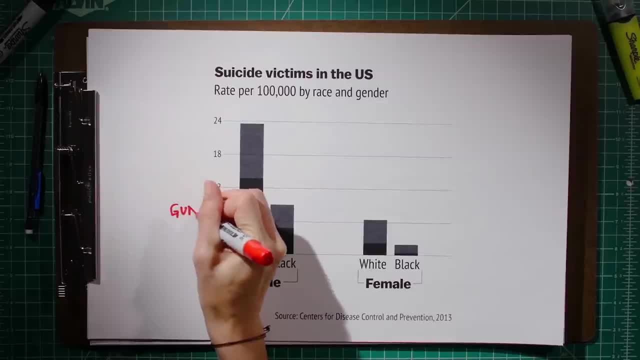 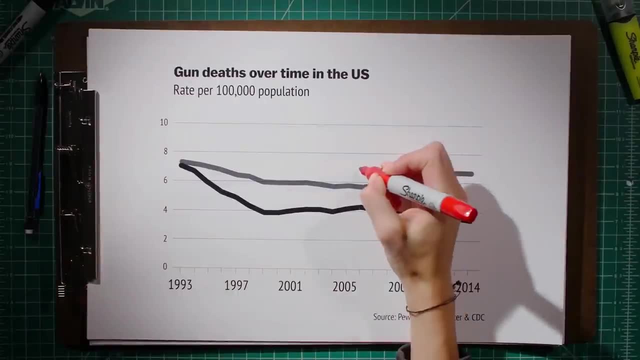 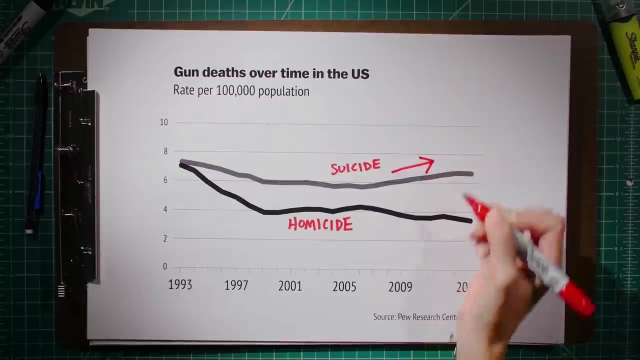 The victims of gun suicides are overwhelmingly men and mostly white, And the rate of gun suicides has been increasing in the US. At the same time, the rate of gun homicides has been decreasing, especially since the 90s, when crime rates in general were higher. 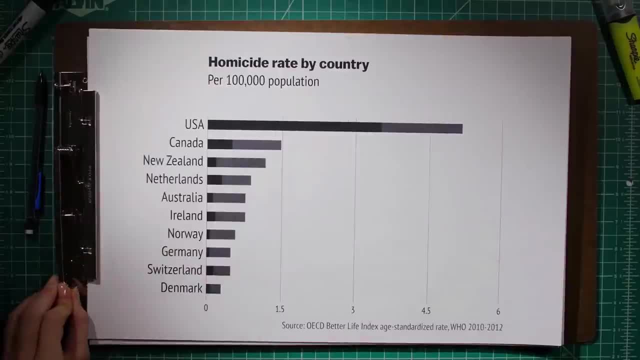 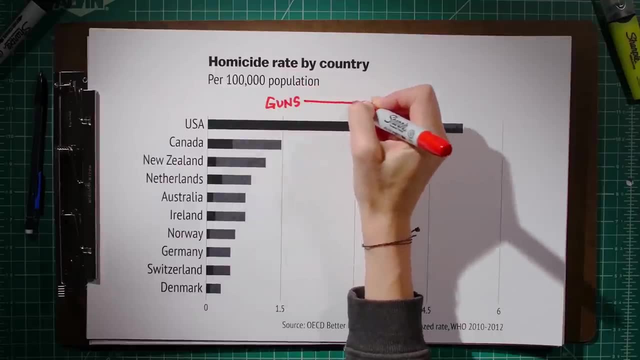 But if you compare the US to other developed countries, it doesn't look like good news. These are homicides adjusted for population size. The US would probably have a higher homicide rate even without guns, But you can see how gun violence pushes that rate far beyond the US. 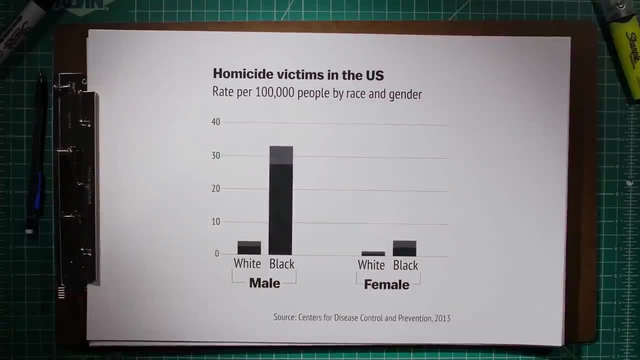 And that's what's happening in the other countries. here The victims of these shootings- they're not the ones you often see on the national news. They're disproportionately young black men. You guys can leave here and go on with your lives, but we gotta go on to empty rooms. Because our children's lives were taken away by people who should not have had guns anyway. One possible explanation is that the US simply has more crime than those other countries. But if you set aside homicides for a moment and look at rates of burglary or assault, 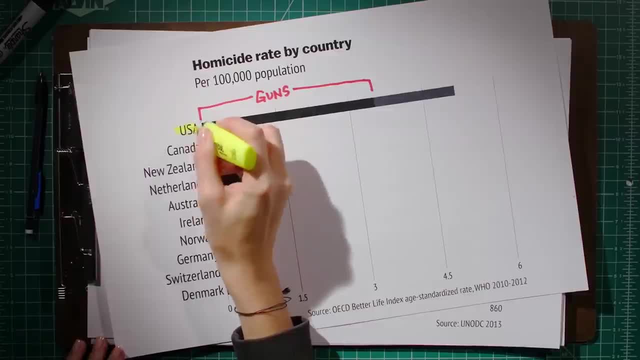 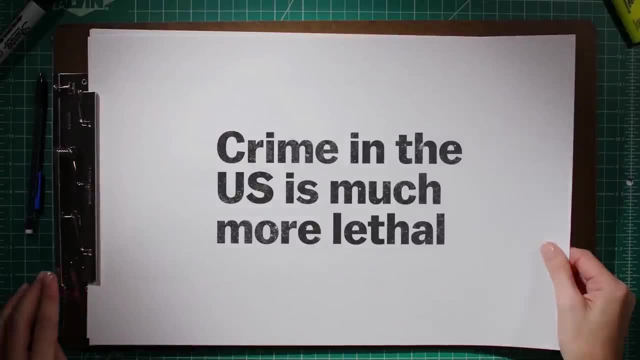 you don't see that same spike that you see with homicide. It's not that America has much more crime. It's that crime in the US is much more lethal. Altogether, the number of gun deaths in the US from 2000 to 2013. 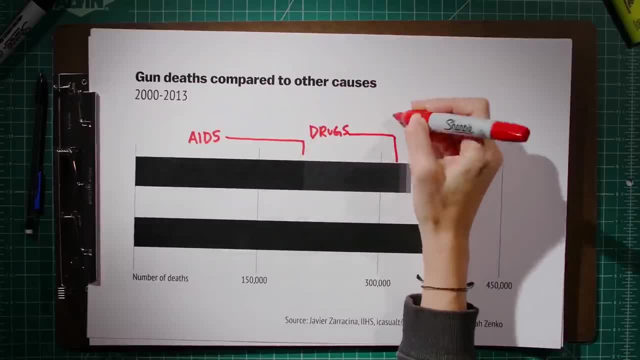 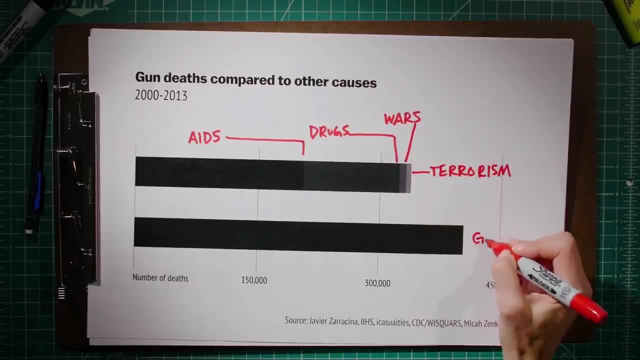 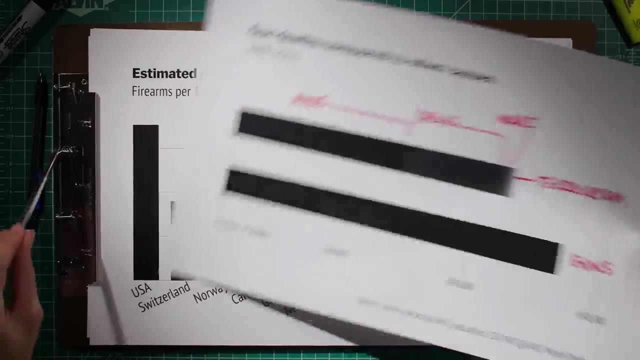 exceeds the number of Americans killed by AIDS, by illegal drug overdoses, the Iraq and Afghanistan wars and terrorism combined, It can be clear by now that this level of gun violence is a uniquely American problem among the developed world, And here's one reason why. 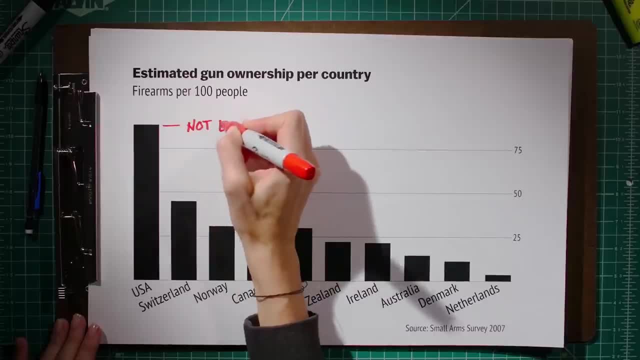 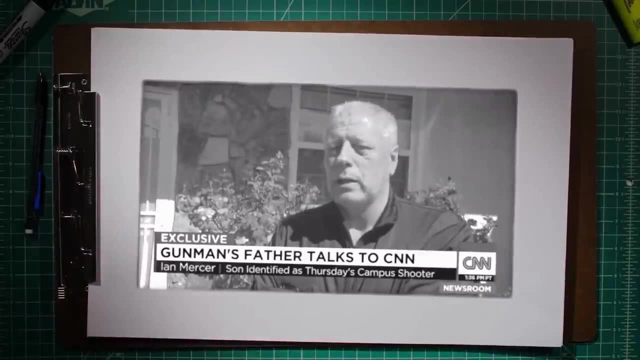 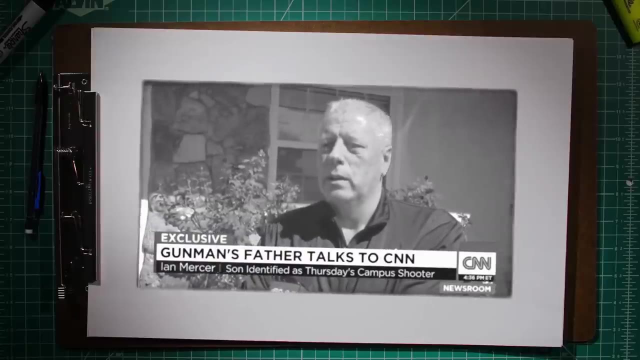 There are a ton of guns in the US. This chart shows the estimated number of guns by country. It's adjusted for population size and it's still not even close. The question that I would like to ask is is: how on earth could he compile 13 guns? How can that happen? If you take a look back at the 10 countries with the highest levels of human development, you can see that it's relatively really easy to get a gun in the US. All of the other countries require a license to purchase most guns. 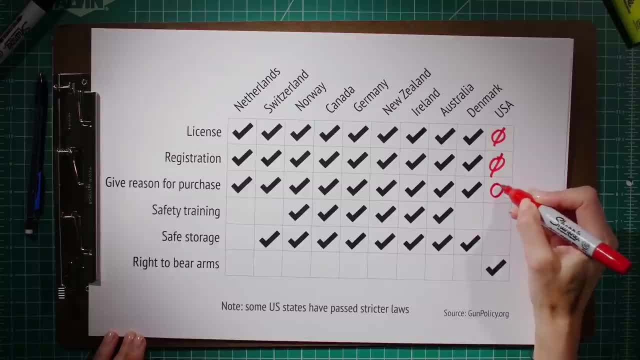 and those purchases are recorded into an official registry. To get that license, people have to state a reason for why they want a gun, And in most of these countries they have to pass a safety test and are required by law to store their guns safely. In part because of its lax laws. there are well over 300 million guns in the US and counting. This chart doesn't reflect that. It doesn't reflect private sales, but it shows the number of background checks which all federally licensed dealers have to run. 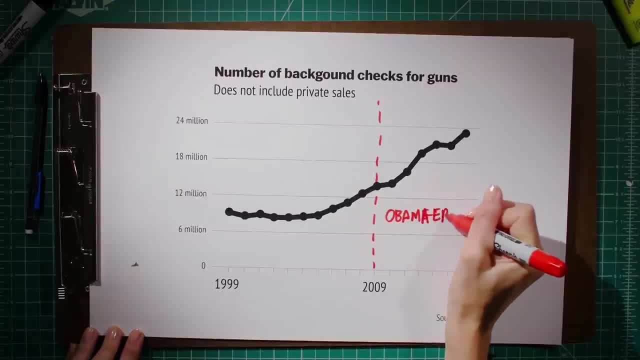 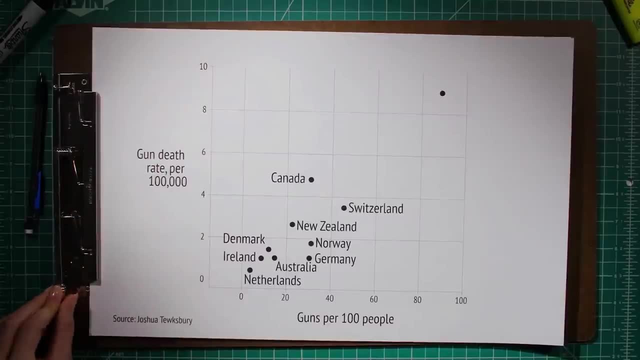 It suggests that the demand for guns has been increasing steeply since Barack Obama took office. So we've looked at gun deaths and at gun ownership. This chart puts them together. It shows that among highly developed countries, the more guns in a country, the more gun deaths. 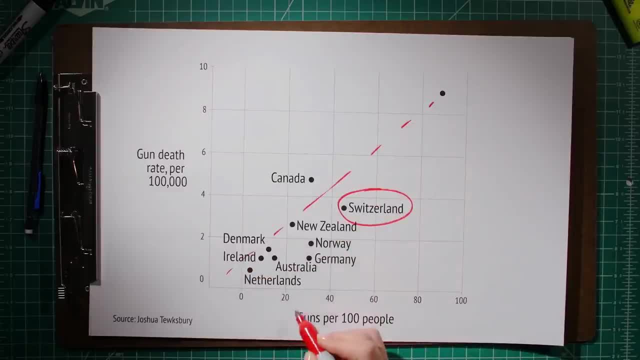 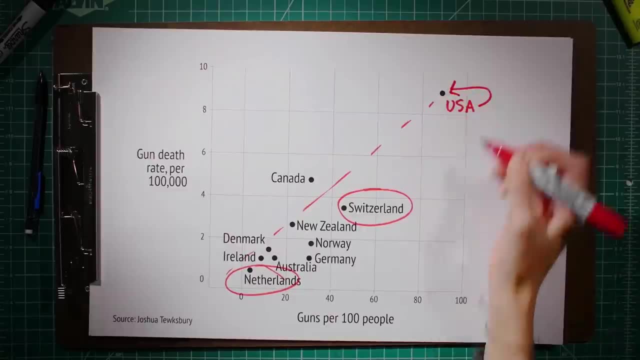 You can see that countries like Switzerland, which have relatively more guns than a country like the Netherlands, also have a higher gun death rate. And here's the US. Likewise, US states with more guns have more gun homicides. There are outliers like Idaho.